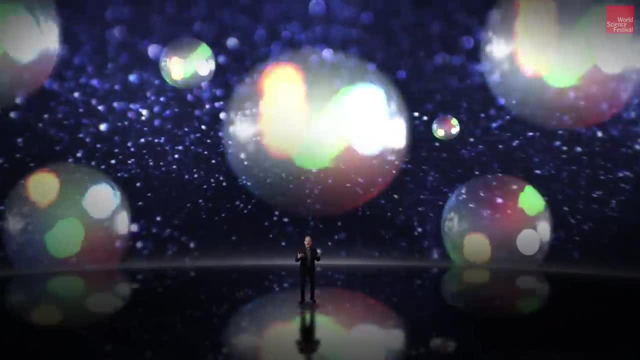 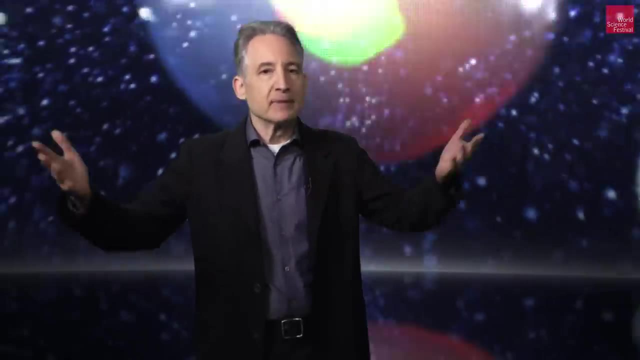 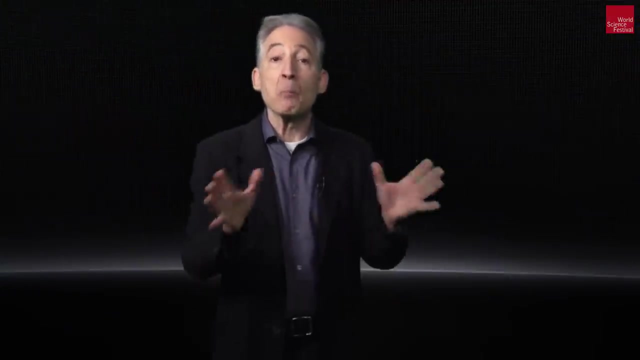 the microworld, the world of molecules, of atoms and subatomic particles, Because in this realm the predictions from Newton's math were they were wrong. The data revealed that new rules were needed to understand the microscopic realm And remarkably, within. 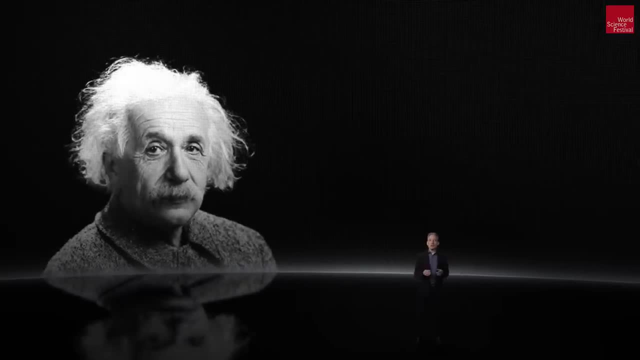 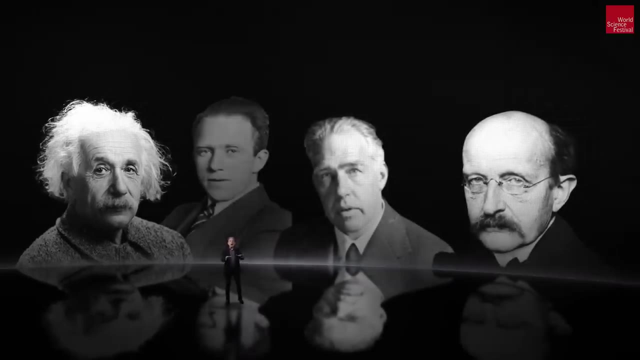 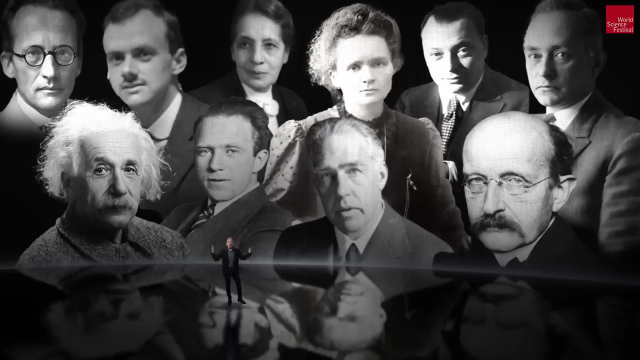 just a few decades, a generation of scientists, including the like of the great Isaac Newton and the likes of Albert Einstein, Max Planck, Niels Bohr, Werner Heisenberg, Erwin Schrödinger, Max Born and many others. this group of brilliant thinkers ushered in a new understanding called 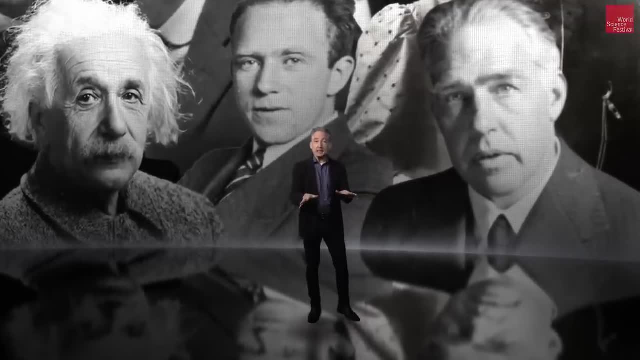 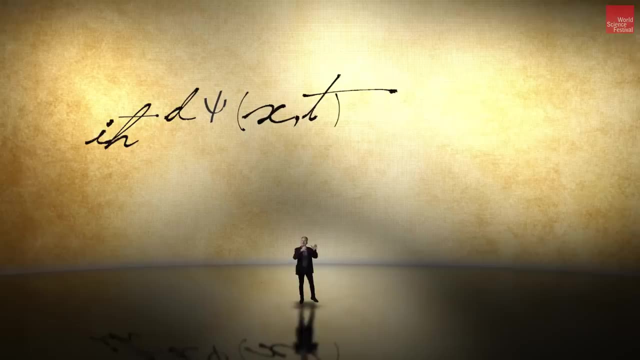 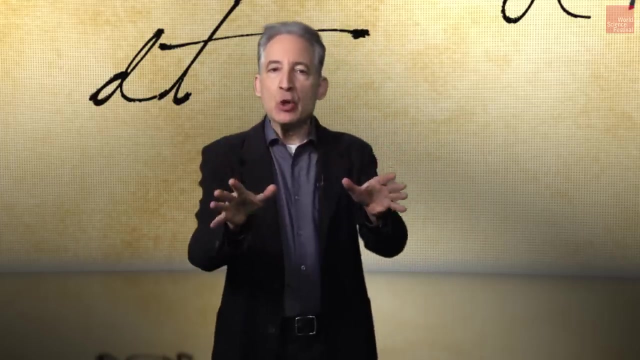 quantum mechanics, Now quantum mechanics. it comes with its own powerful mathematical formulation, But again one can grasp the central new idea of quantum mechanics, and even without the math. Whereas Newton said: tell me how the world is now and I will tell. 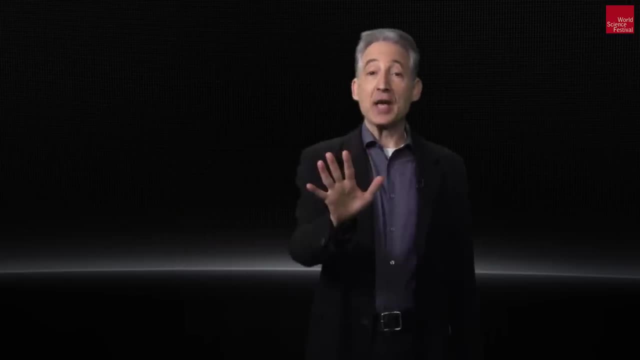 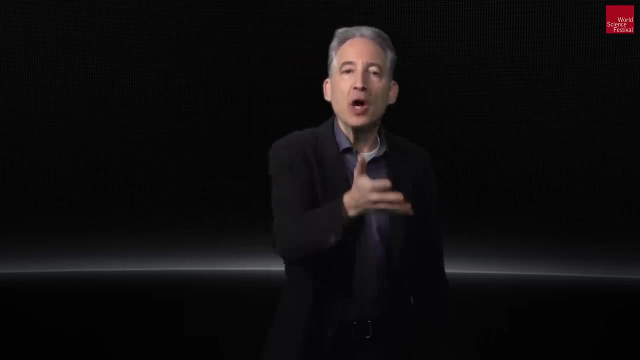 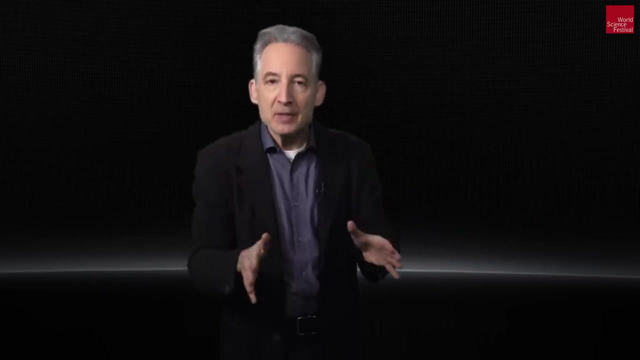 you how the world will be tomorrow. Quantum mechanics says: tell me how the world is now and I'll tell you the probability that the world will be one way or the other tomorrow. And according to quantum mechanics, these probabilities provide the deepest and most. 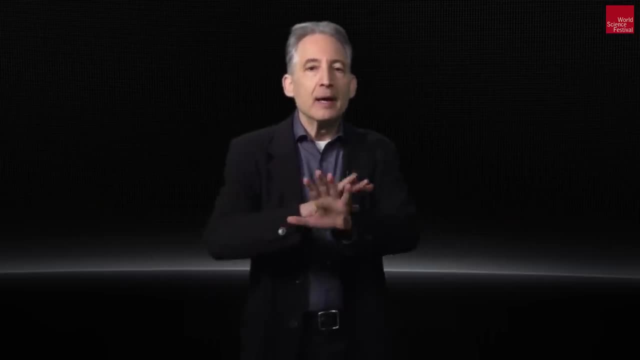 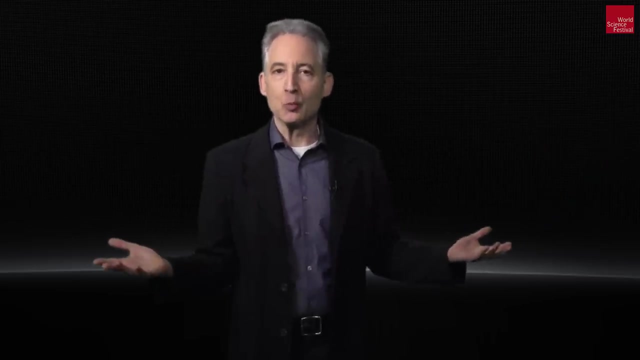 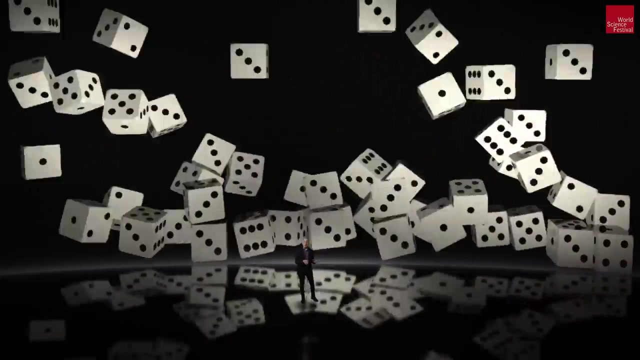 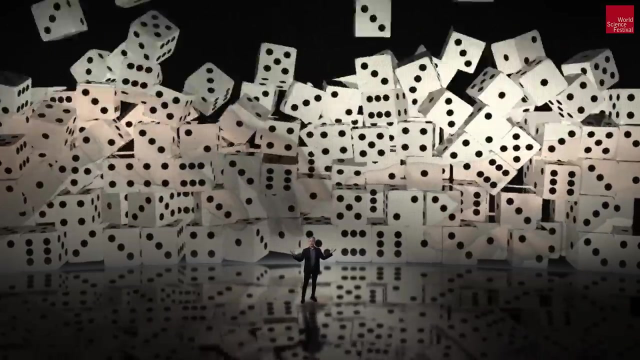 precise description of the physical unfolding. Gone completely gone, according to quantum mechanics, was the rigid certainty of the classical world. Now much has been made of Einstein's resistance to the probabilistic nature of quantum mechanics. the famous and frequently quoted God does not play dice. 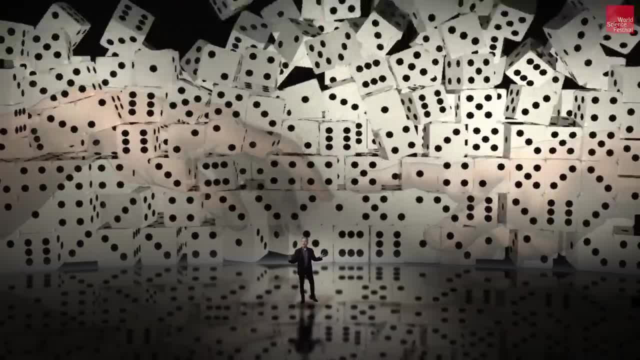 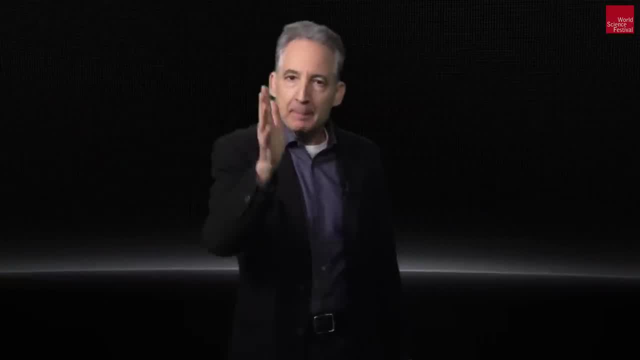 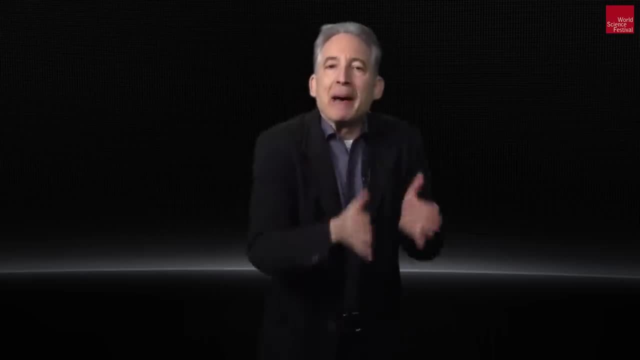 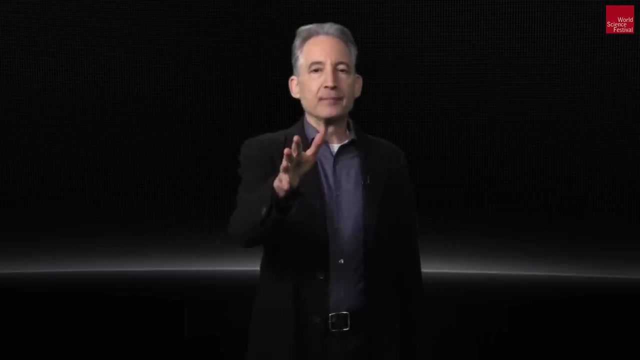 But Einstein did not deny that quantum probabilities provided a spectacularly accurate description of the microscopic realm. Instead, he firmly believed that quantum mechanics was only a provisional theory, one that would ultimately be replaced by a deeper understanding that would not rely on probabilities, And, toward this end, Einstein worked tirelessly to expose. 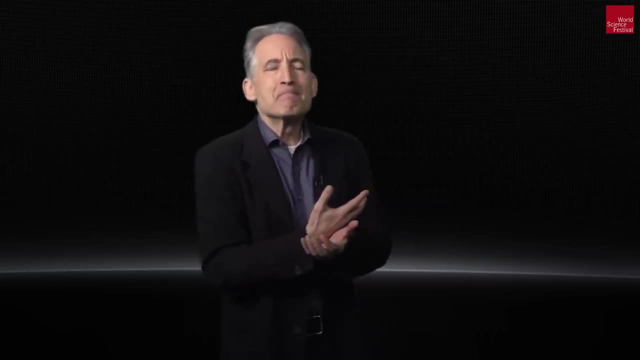 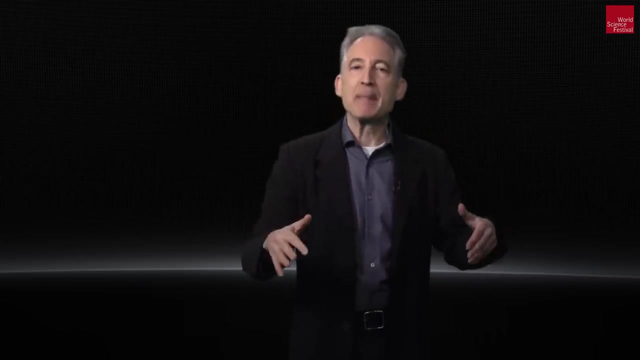 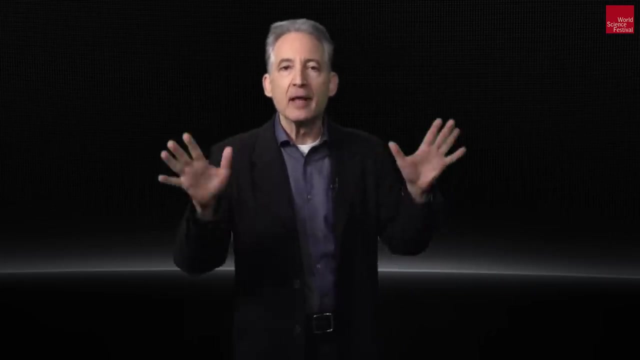 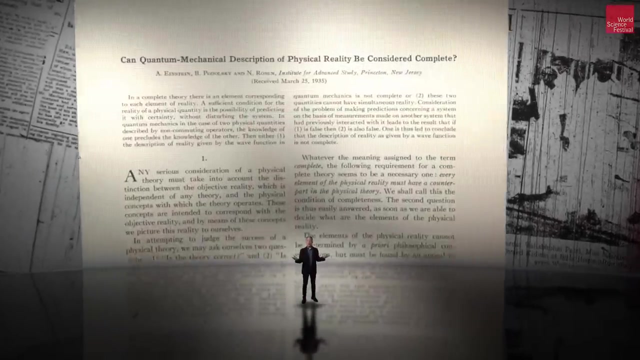 qualities of quantum mechanics that he hoped would be so obviously unacceptable, so counter-intuitive to any reasonable person's expectation of how the world works, that everyone would have to agree with his view that quantum mechanics was not the final story. In 1935, with two colleagues, Boris Podolsky and Nathan Rosen, Einstein believed he had 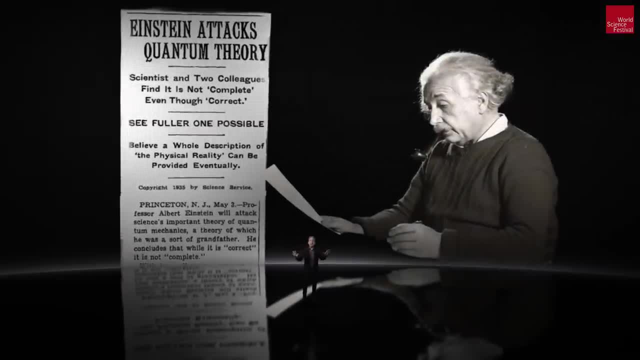 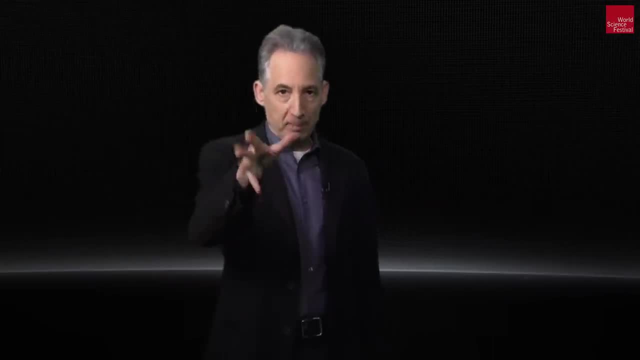 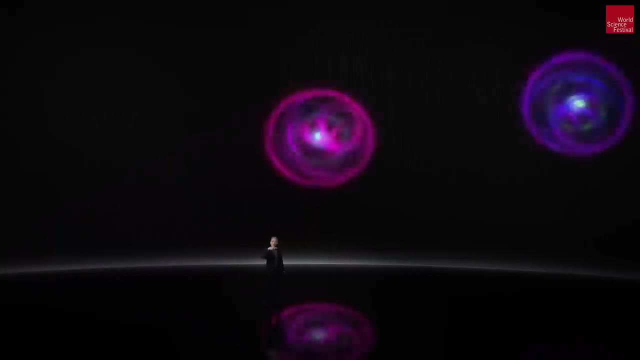 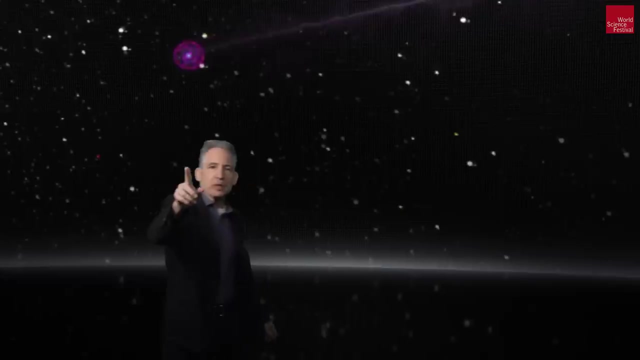 finally found the ultimate quantum mechanical Achilles' heel, with a property inherent to quantum mechanics called quantum entanglement, Briefly put, Quantum entanglement. Now, Einstein and his colleagues found that, according to the math of quantum mechanics, If two objects interact and then widely separate a subsequent measurement on one, 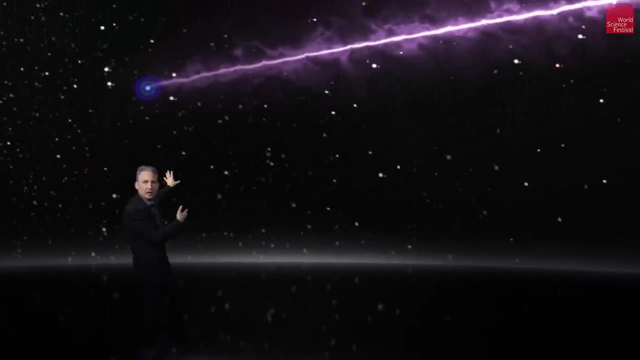 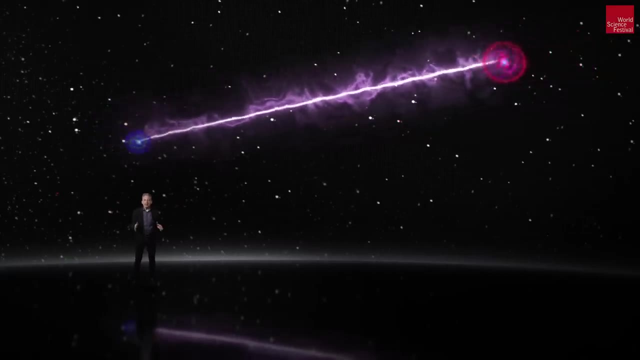 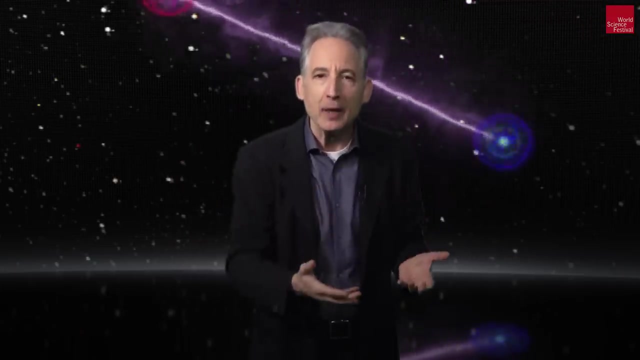 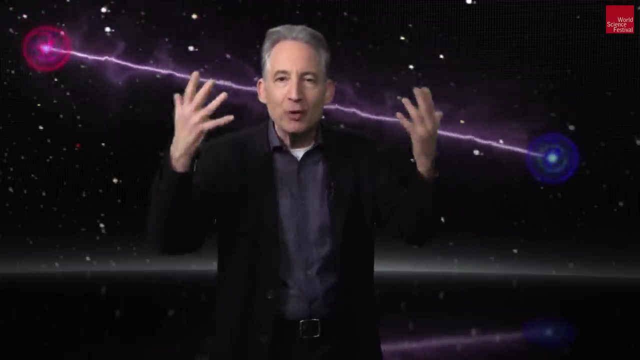 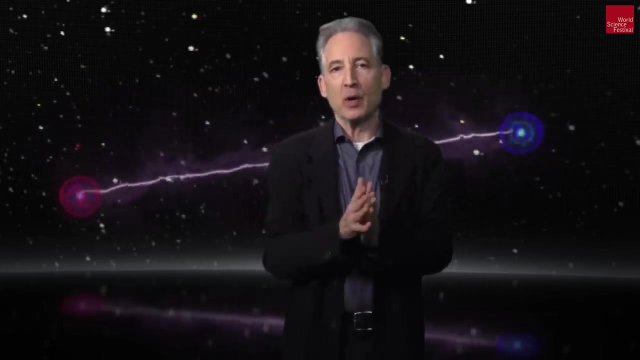 of those objects revealing one or another quality would have an instantaneous influence on the other object, regardless of the distance between them. Einstein called this strange connection. he called it spooky, spooky action at a distance, and it troubled him deeply. his, his straightforward, intuitive belief was that widely separated objects are independent of one. 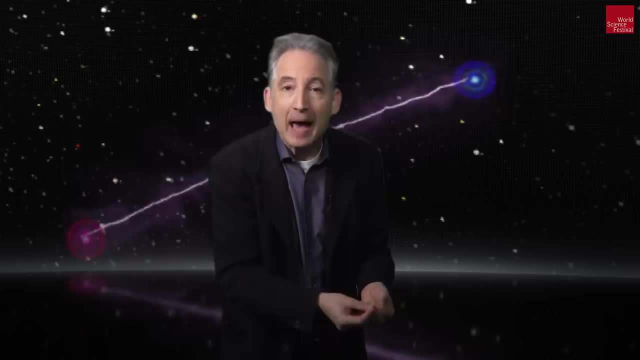 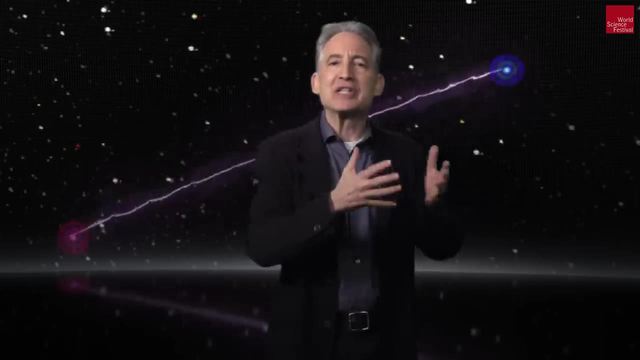 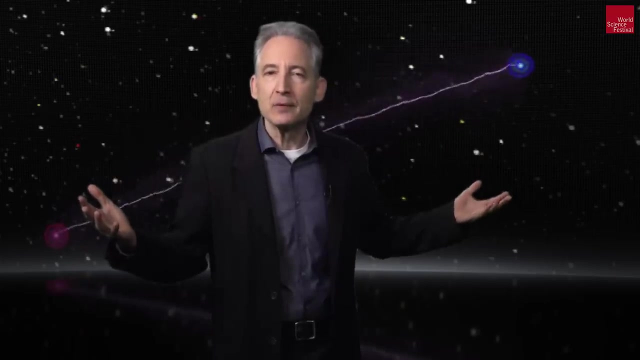 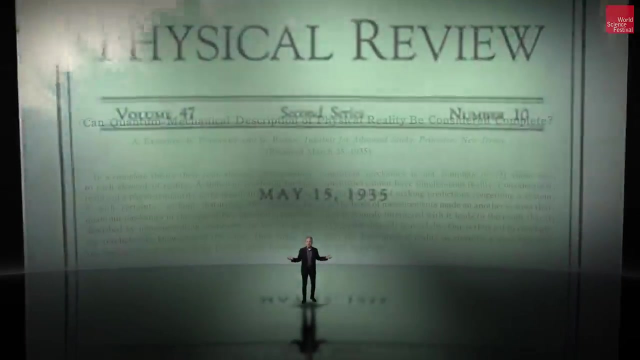 another. but quantum entanglement seemingly denied that by providing an invisible quantum connection capable of linking the distant objects together or, as the name says, entangling them. einstein could not accept this quantum view of reality, and so he concluded that something had to give. quantum mechanics could not be the full and final story. that's the upshot of the 1935. 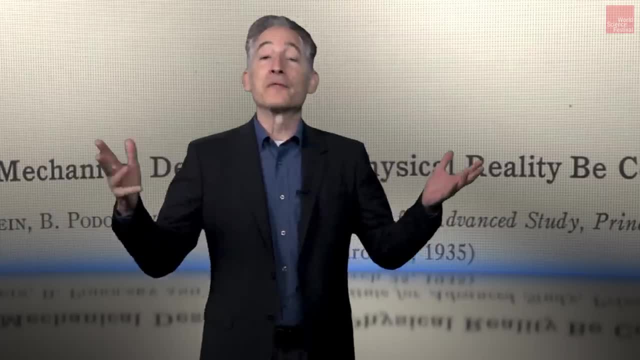 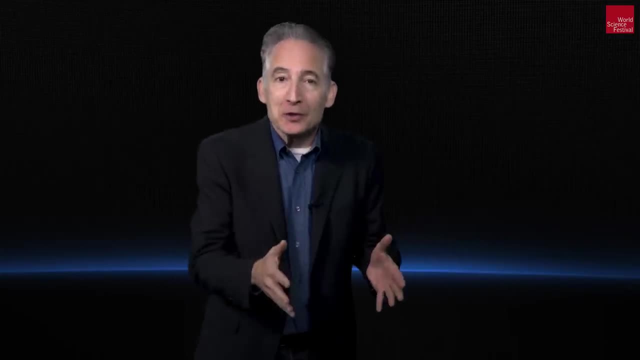 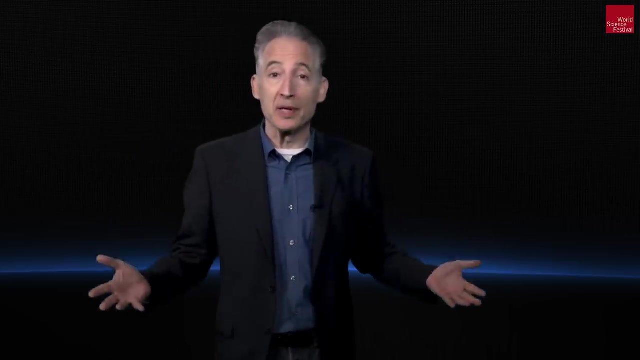 so-called epr paper. now for years no one paid much attention to the epr resolution of quantum mechanics. it was only just a short, and clear Cummings University result, mostly because quantum mechanics worked and, moreover, no one could see a way to test Einstein's speculation that quantum mechanics would one day be replaced by a deeper understanding. 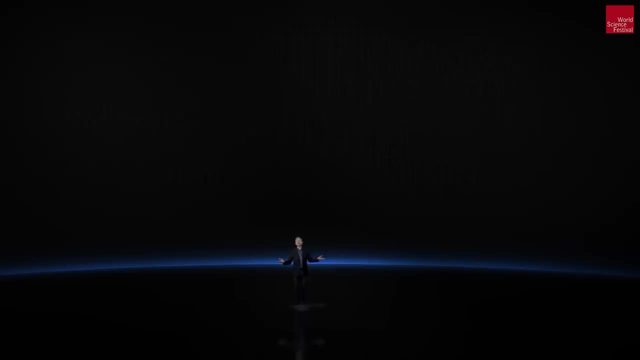 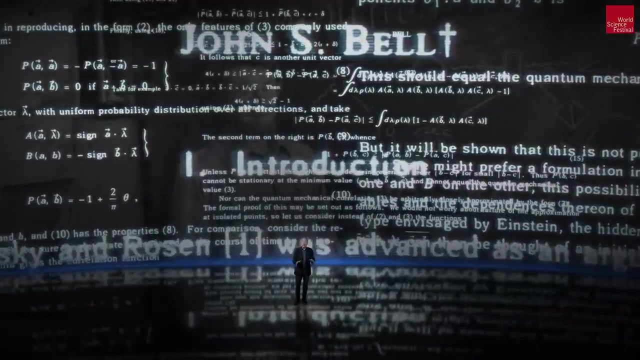 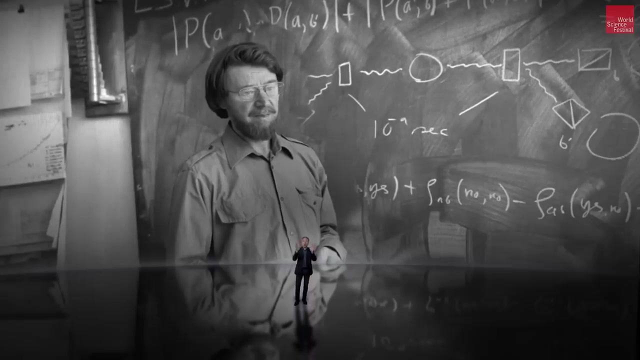 that would not need probabilities. That is until 1964, when a physicist named John Stuart Bell proved mathematically that there was a way to test Einstein's more conventional view of reality, that is, to test his view that particles always have definite features and there's no spooky connections, no quantum. 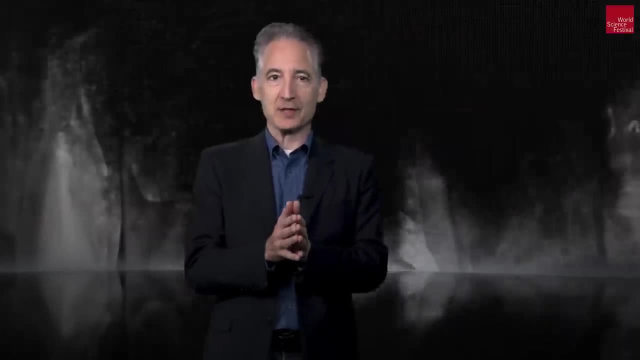 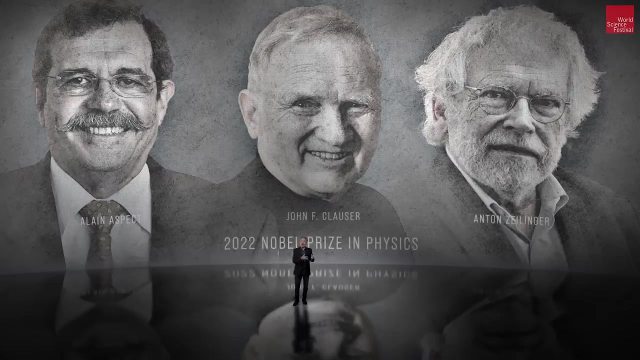 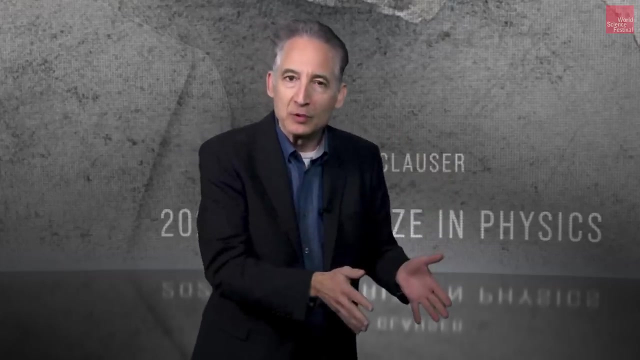 entanglement, And this year's Nobel Prize in Physics has been awarded to Alana Spey, John Clouser and Anton Zeilinger, whose collective works have carried out that test, establishing to most people's satisfaction that Einstein's conventional view of reality is ruled out. 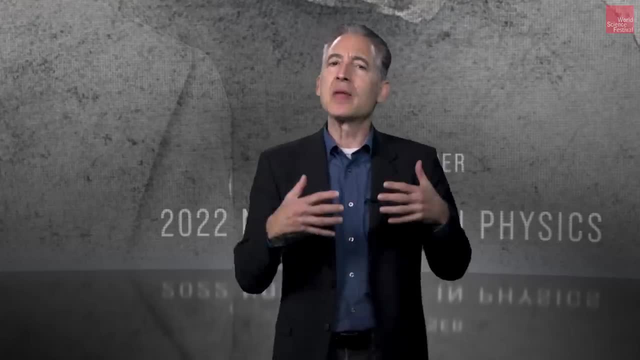 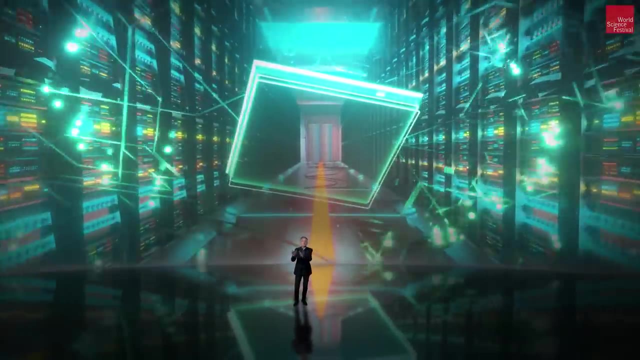 that quantum entanglement is real and more than that, have shown that quantum mechanics and entanglement can be solved And that they can be leveraged for applications ranging from quantum computing to quantum teleportation: spectacular results that have both changed our view of reality and whose 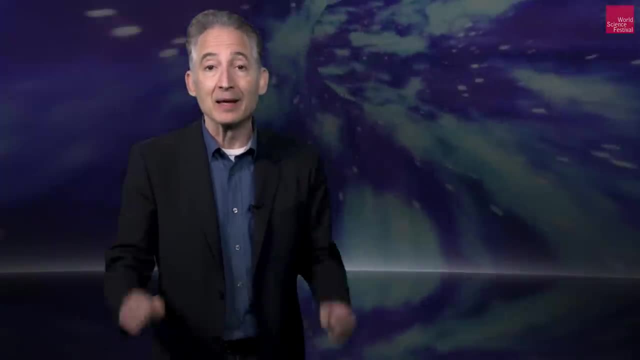 technological implications are both exciting and profound. 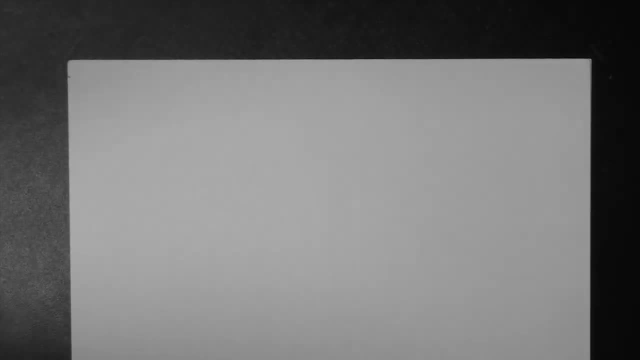 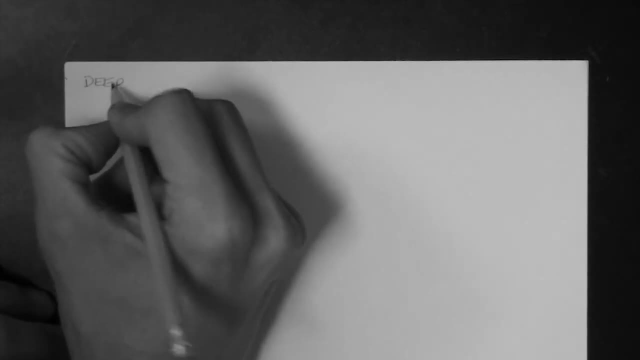 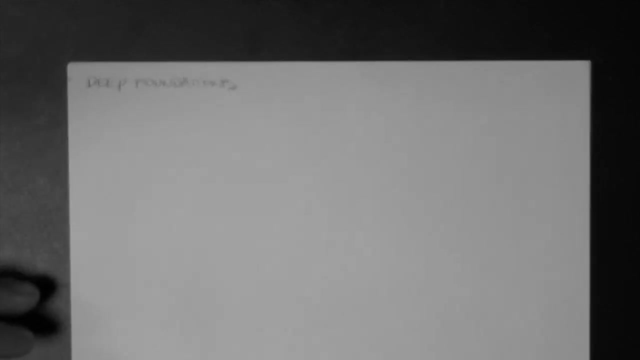 Okay, this is a quick and informal video about deep foundation types. okay, Deep foundations, All right. so deep foundations are essentially, in quotes, called piles. Now we'll see in a second what the actual definition of a deep foundation is, but in general, the type of deep foundations. 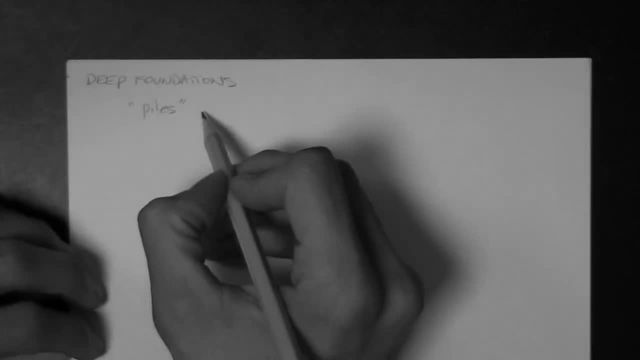 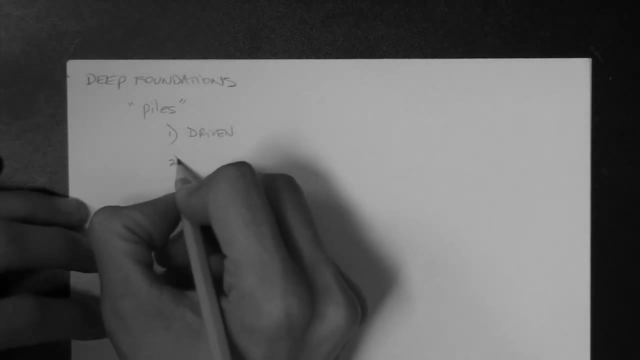 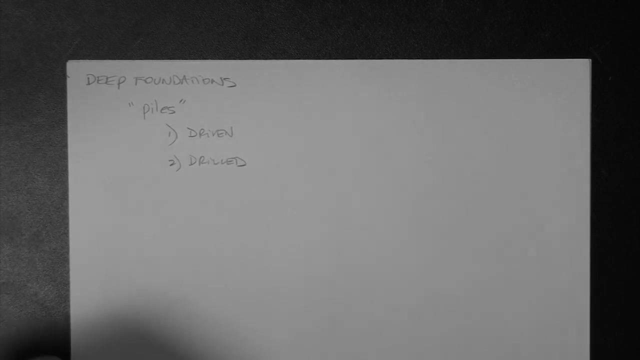